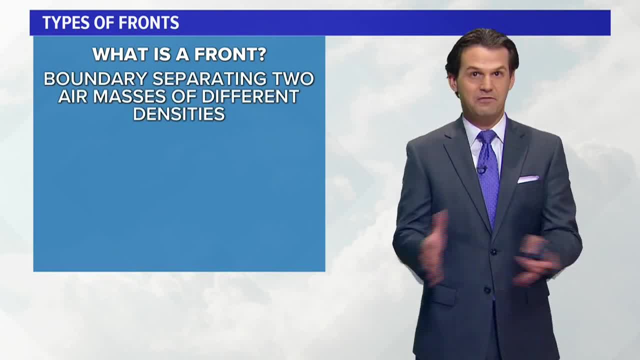 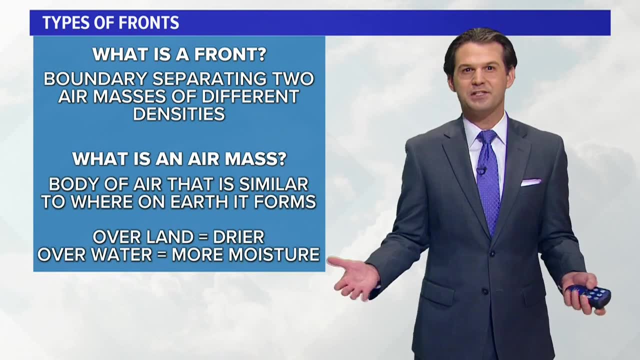 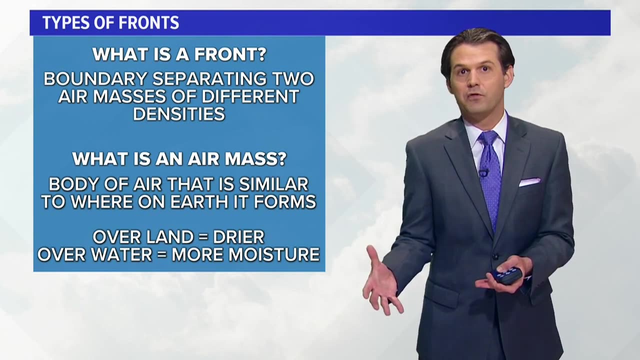 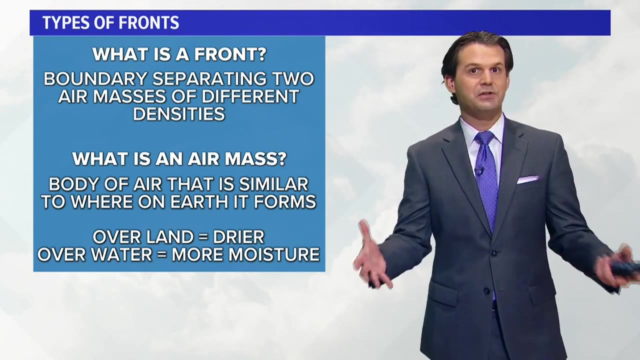 warm front. Well, it's a boundary separating two different types of air masses that have different densities. So you may be wondering: well, what's an air mass? Well, an air mass is just a body of air that is similar to where it forms on the earth. If that air mass forms over land, usually it's drier. If it forms over water, usually it has a little bit more moisture. Think about, you know, one day when it's dry and warm outside, that's a certain type of air mass, And then maybe the next day it's kind of damp and rainy. Well, that would be a different air. 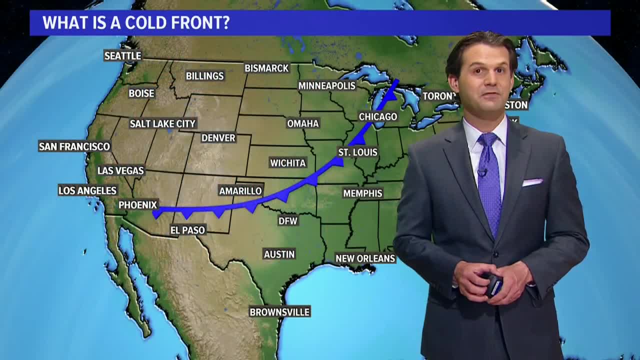 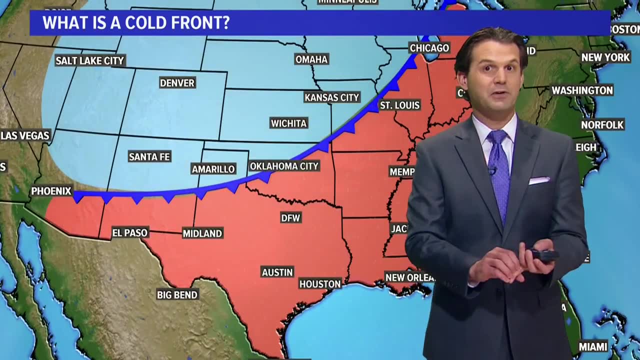 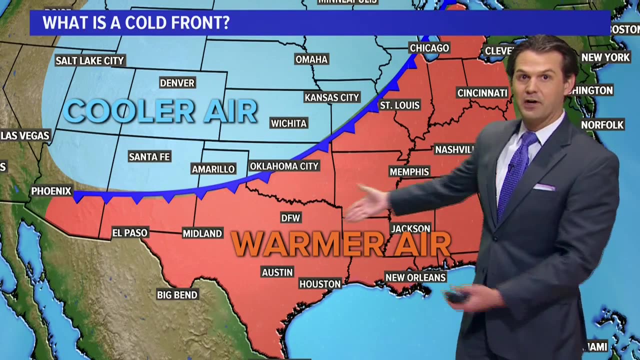 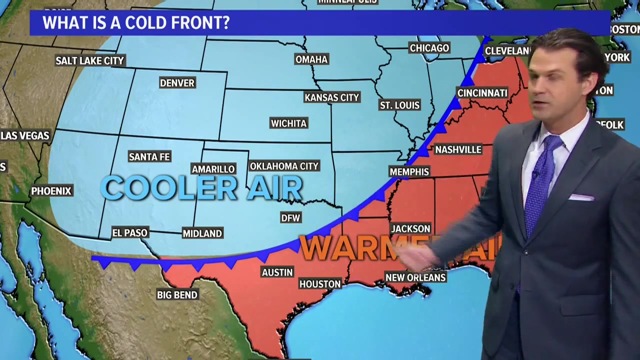 mass That kind of moved in, maybe because one of these types of fronts moved overhead. So first let's talk about a cold front, probably the most common type of front that we see here in North Texas. Remember, it's a boundary that separates two different air masses. So here they are. You got cooler air behind the cold front, warmer air at ahead of the cold front. here in North Texas DFW area We're stuck in that warmer air, But what happens is that cold front moves through, cooler air moves into North Texas. Now you can tell which way the front is moving, by which side the little symbols are on. So here the 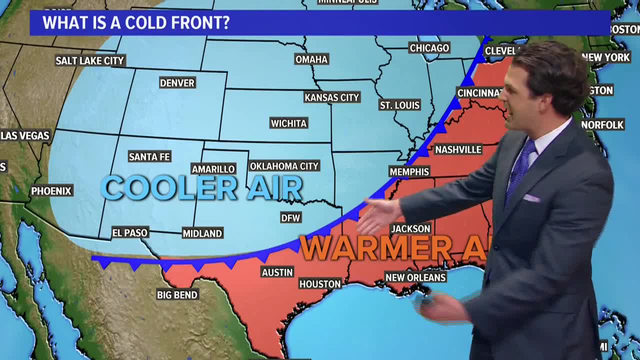 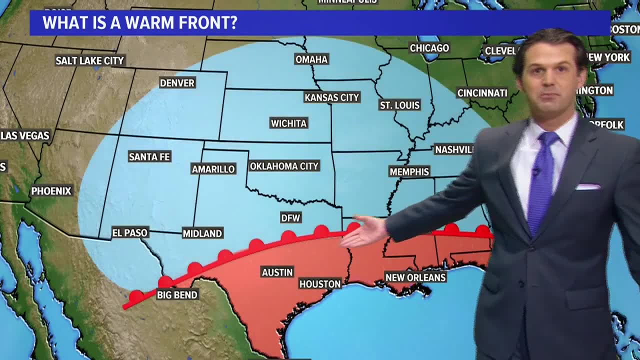 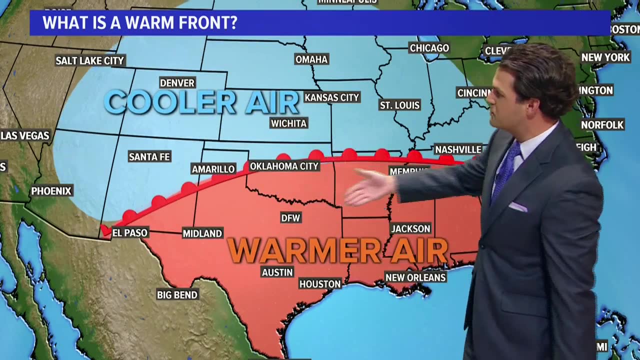 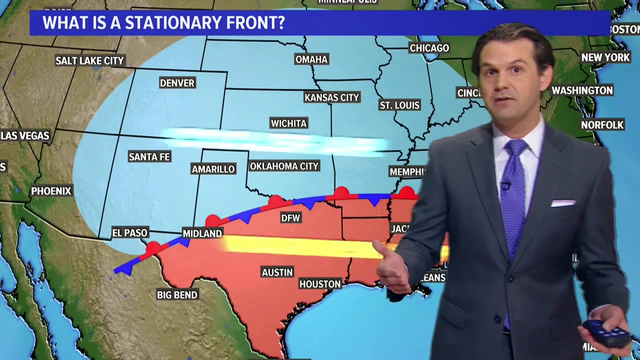 triangles are on kind of the southern side, or you know downward side of that cold front, means it's moving to the south. Well, what about a warm front? Remember it's a boundary that separates two different air masses. They're still cooler air and they're still warmer air, But this time- remember where the symbols are- The warmer air is moving into North Texas and the cooler air gets pushed a little bit farther to the north. Now that stationary front is a separation of the cooler air and warmer air, but it's stationary, It's just not moving. So it's not moving. 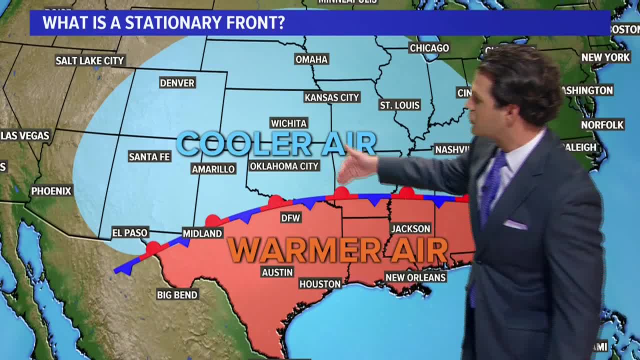 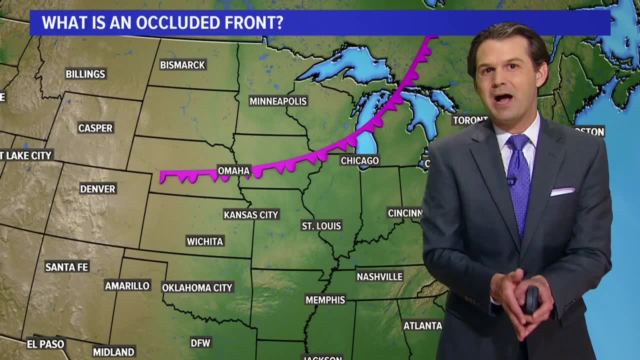 That's a boundary, not, you know, mild front or something like that. There's still cool air to the north, warmer air to the south, but it's just not really moving. now An occluded front, this one, the most complicated, and we're not going to see. 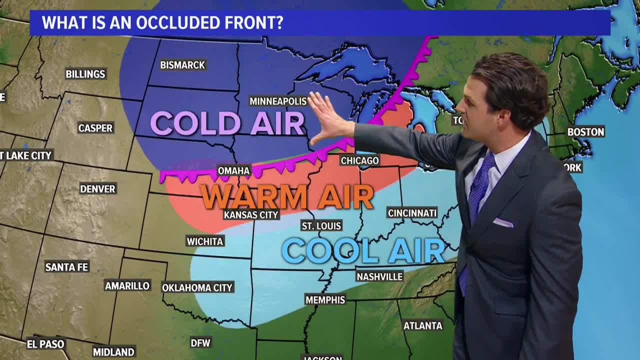 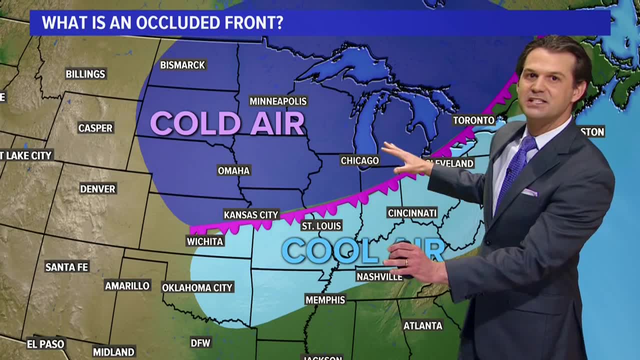 these hardly ever in north Texas. Basically it's a boundary between really cold air- There may be a sliver of warm air and then a little bit of cool air, And as that occluded front drifts to the south, it kind of erases. 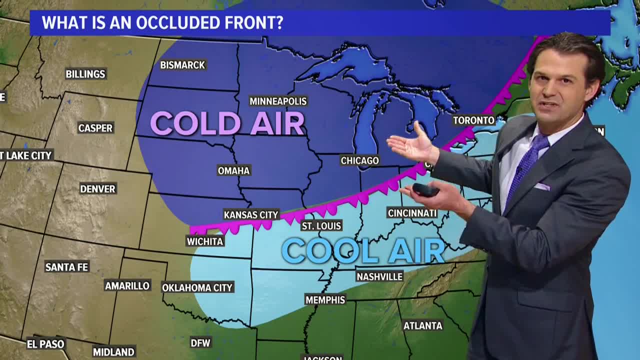 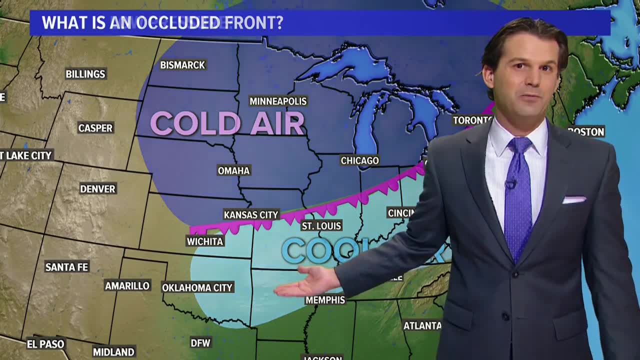 the warmer air or lifts it up higher into the atmosphere. So then the occluded front becomes a boundary between kind of more cold air and cooler air. Like I said, those are a little complicated and we hardly ever see them here in north Texas. Now what about low pressure? low pressure, That's.